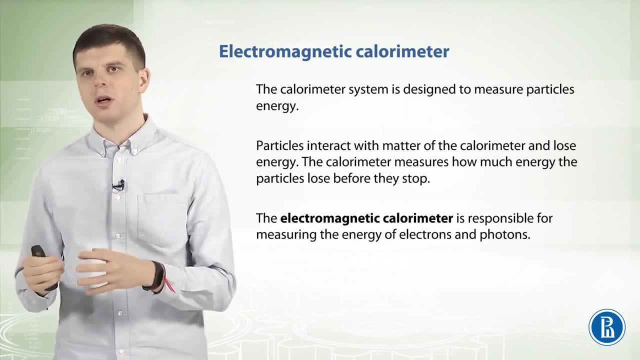 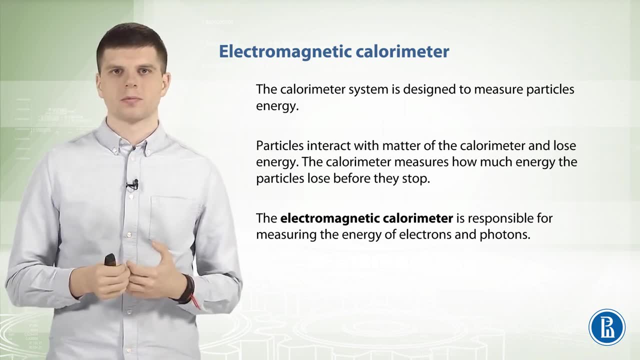 So the colorimeter system is designed to measure particle energy. Particles interact with much matter of the colorimeter and lose their energy. The colorimeter measures how much energy the particles lose before they stop. Let's start from the electromagnetic colorimeter. The electromagnetic 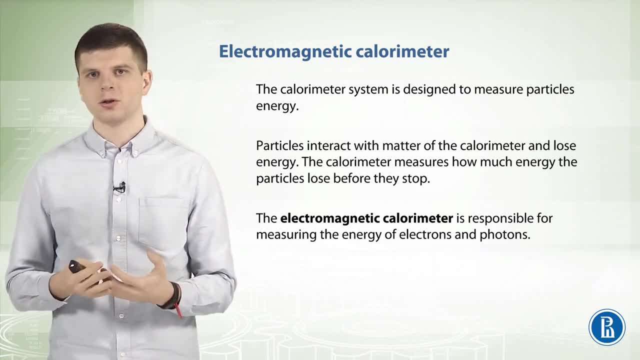 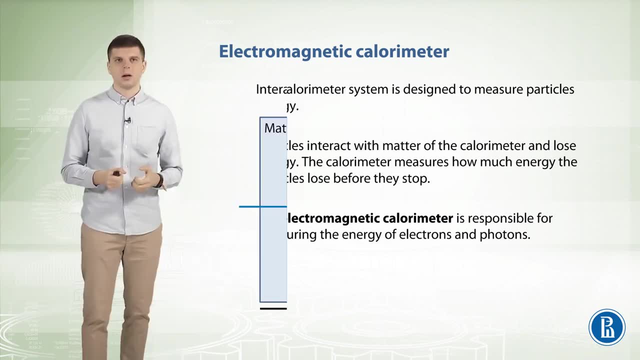 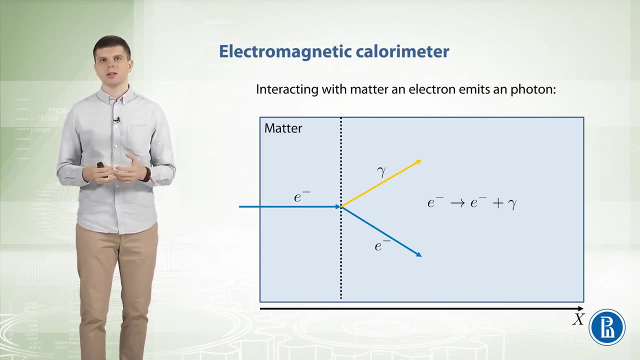 colorimeter is responsible for measuring the energy of electrons and photons. Consider how the electromagnetic colorimeter works. Suppose an electron flies into the colorimeter. Interacting with the matter, the electron emits a photon. Interacting with the matter, the electron emits a photon. 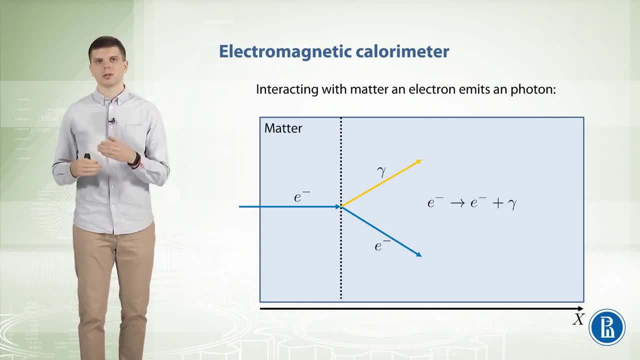 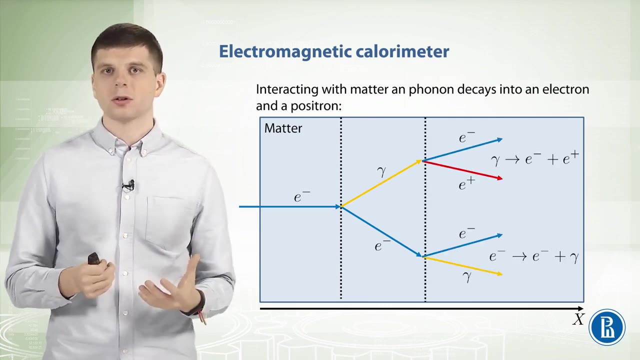 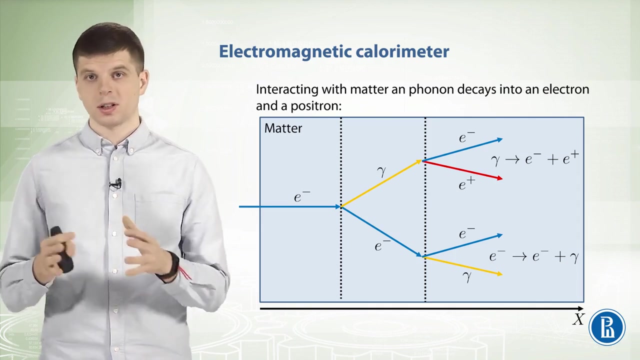 The electron loses some energy as it passes through the person. The electron bonded into an individual particle, thus transforming into a fragment. The blue calorimeter has this curve: Theumed, proton becomes theамor and changes its own direction, losing some energy. After this first step, we have two particles and some of their. 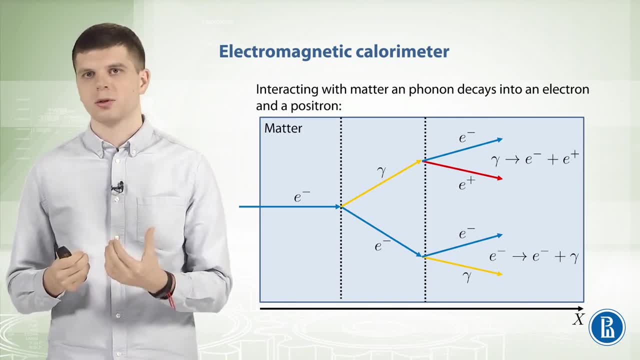 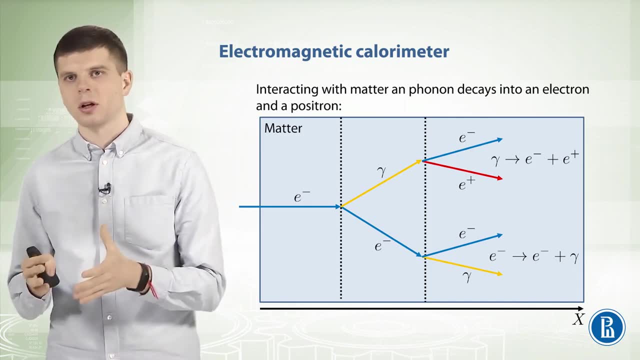 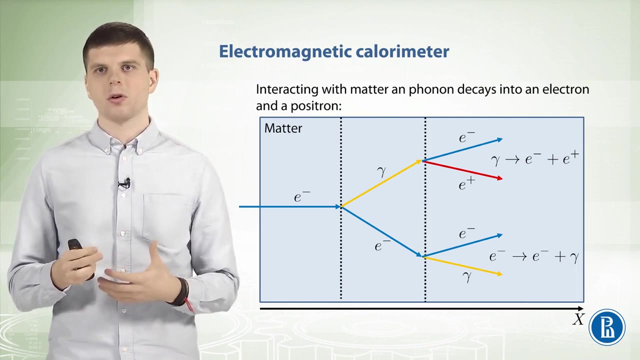 energies are equal to the energy of the original electron. vemos ك�먼. At the second step, the photon interacts with the matter, changes its own direction and lose energy. So there are four particles and energy of the region. electron is distributed on these particles. In other words, with each step, the number of 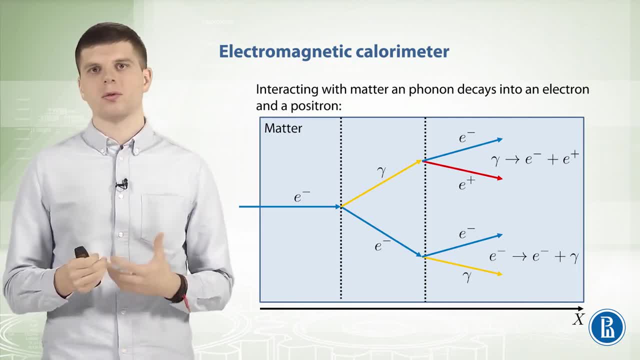 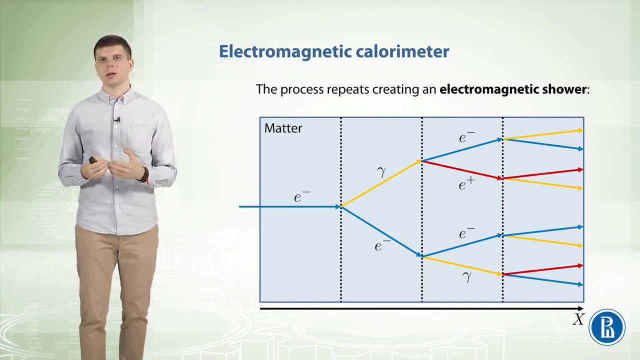 particles increases and energy of each of these particles decreases. This process repeats a lot of times and creates an electromagnetic shower. During this process the number of particles exponentially increases and some of their energies is equal to the energy of the origin electron. So energy of particles in the shower exponentially drops with each step of the process. 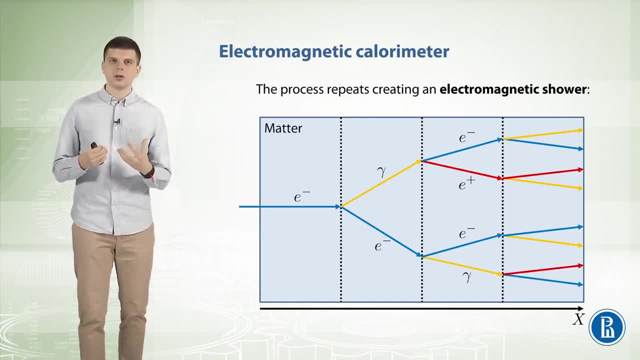 Moreover, each step takes in average the same distance in the material of the detector And as a result, particle energy in the electromagnetic shower exponentially drops with length of the shower. Let's formalize this So: energy of a particle in the electromagnetic shower. 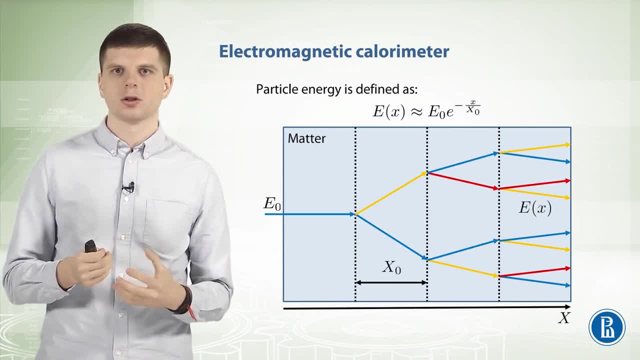 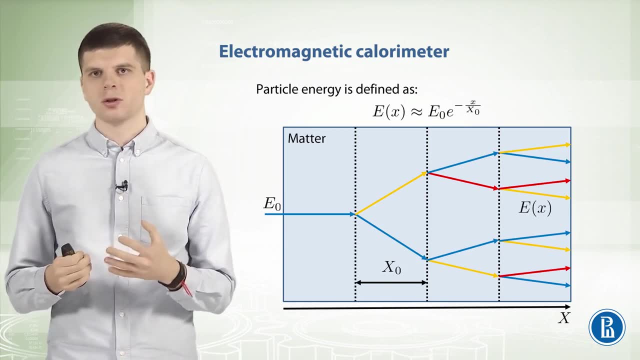 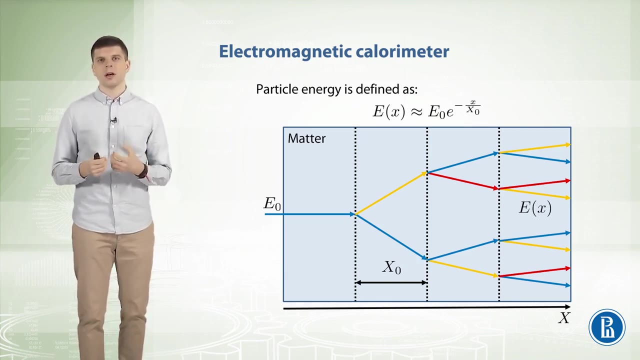 exponentially drops with its coordinates in the shower and proportional to the starting energy. E0 for the origin particle, as shown on the slide. In this equation, xx0 represents average size of one step of the electromagnetic shower production, And this value depends on material used in the colorimiter. 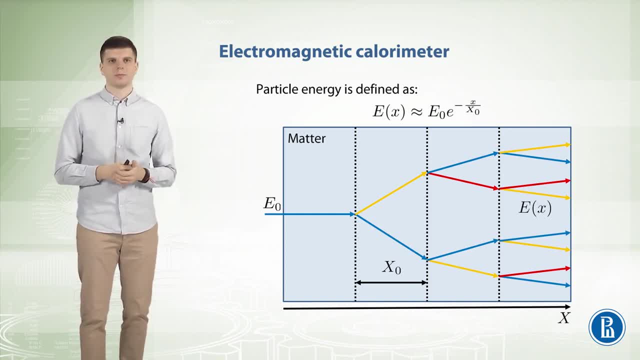 The more dense material – the smaller this value. This equation allows to estimate the shower pressure in a given total of E0.. So from this amountую FcM we get e0, and from E0, E0, Sf, C0,, C0, Цb and C0 Vader. But we don't know how great is the time of the frequency part in Obrigan's answer, Because we don't even know how it is the stretch meter and what is the 차 jegger of North cross Як Zi there. so it helps to find out what order here, but we gna to do an evaluation about it'. 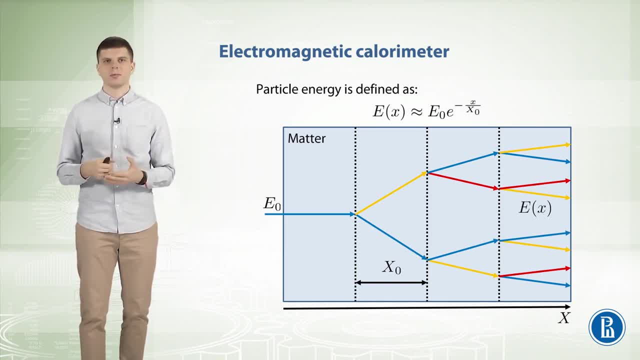 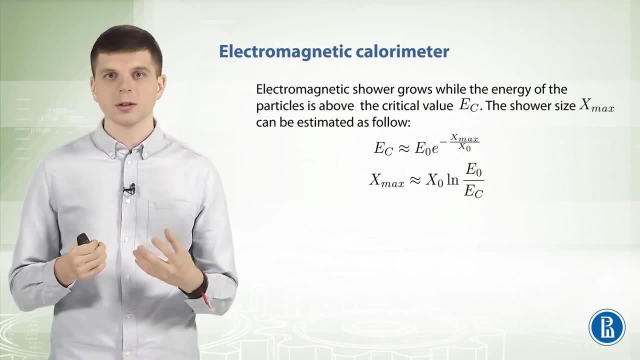 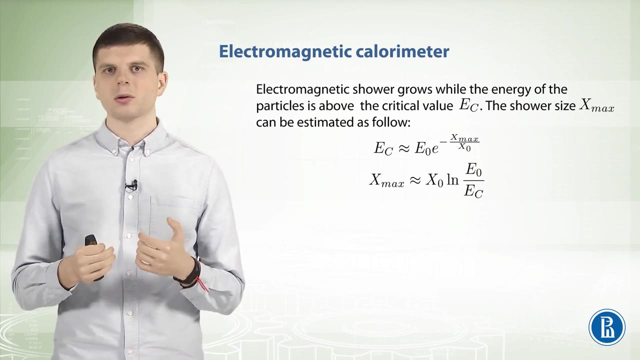 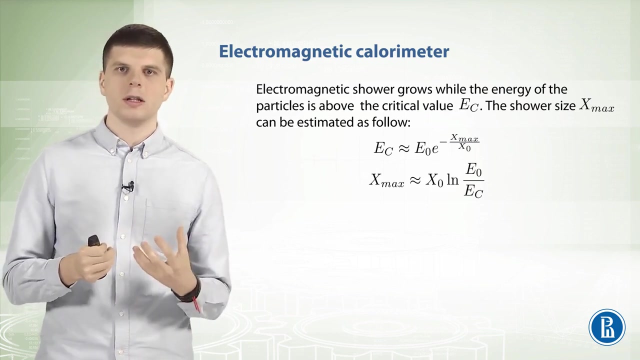 size and number of particles in it. Let's consider that Electromagnetic shower grows while the energy of the particles in the shower is above the critical value Ec. The shower size x max can be estimated as shown on the slide. The critical energy Ec as well as x0 in the equation are: 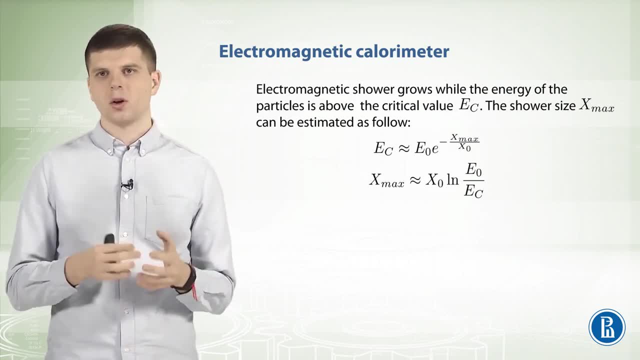 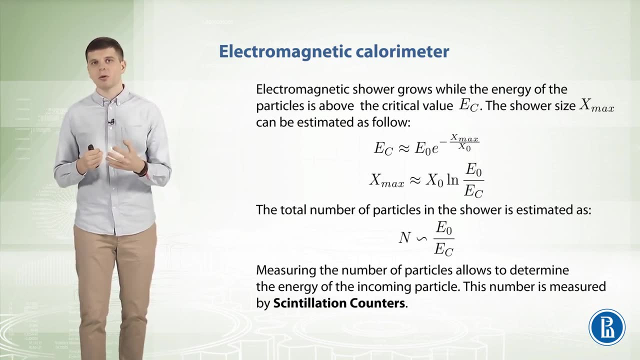 defined by the material of the calorimeter and width of the calorimeter, and selected to be larger than the length of the shower. The total number of particles in the shower is estimated as follows: It's proportional to the energy of the origin particle E0 and inversely depends on. 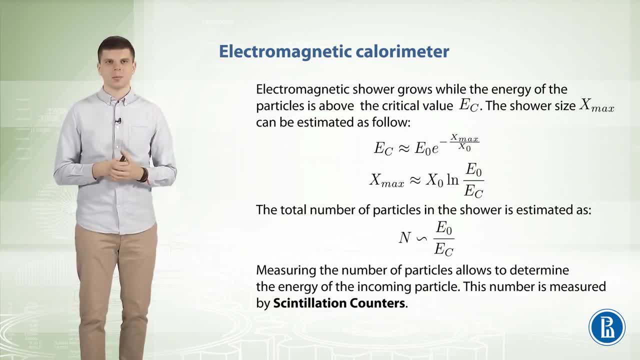 the critical energy Ec. Measuring the number of particles allows to determine the energy of the incoming들이uelocal puede constraint Cartical energy between the particles of the shower variation population is two times the energy of the accelerating cream. That is to say that thePs, которое 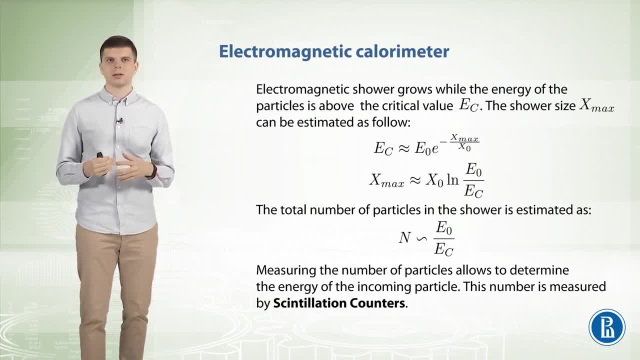 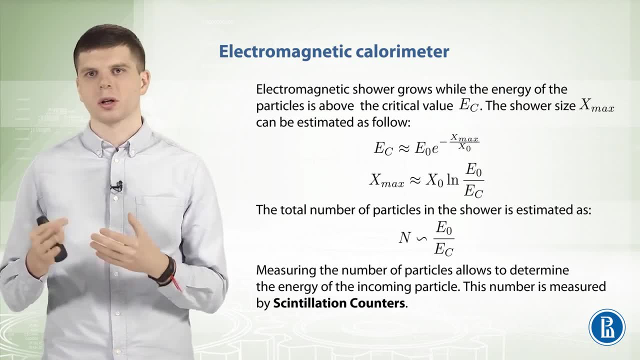 not the number of particles it can be dirty created. Energy of particles results in the energy of brill, 왜력GEc particle. This number is measured by scintillation counters. Their signal is proportional to the number of particles flies through the counters. Consider: 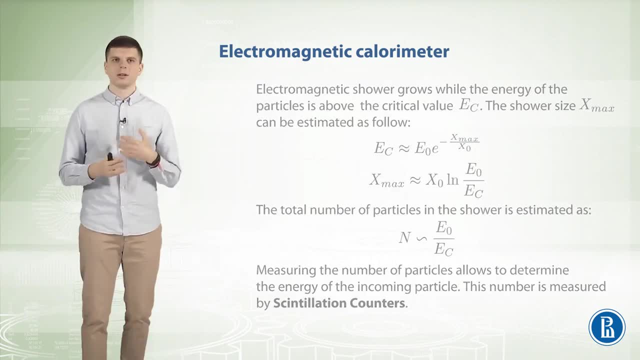 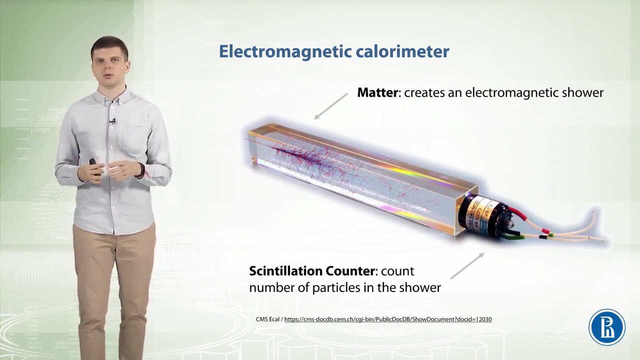 composition of the electromagnetic colorimeters In the high-energy physics experiments. electromagnetic colorimeters consist of a lot of crystals shown on the slide. The crystal creates an electromagnetic shower and length of these crystals is selected to be larger than expected size of the shower. The 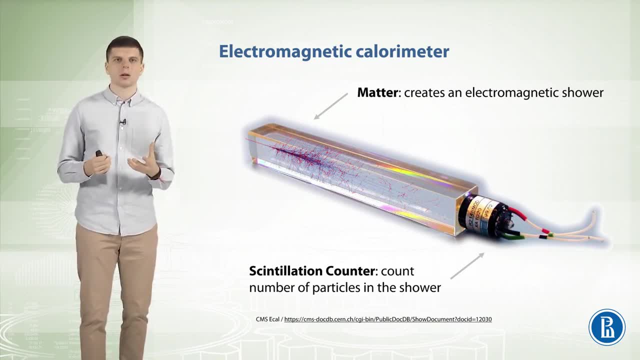 crystals are transparent because a lot of particles in the shower are photons. Also, there is a scintillation counter after the crystal. It counts the number of particles in the shower. This number depends on the incoming particle energy and this dependence is estimated due to the number of particles in the shower. 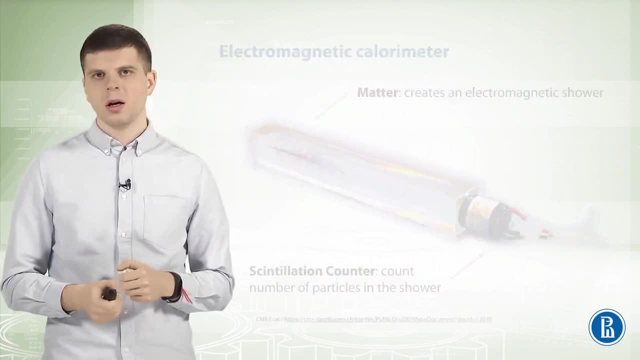 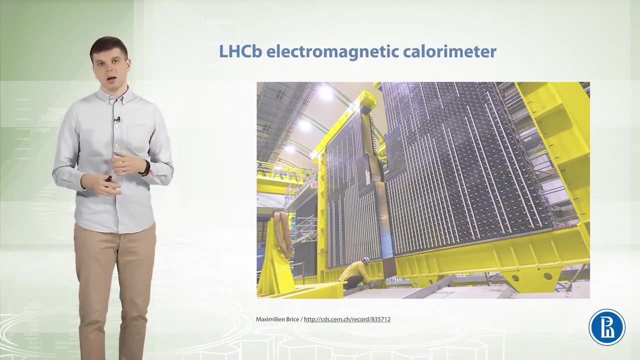 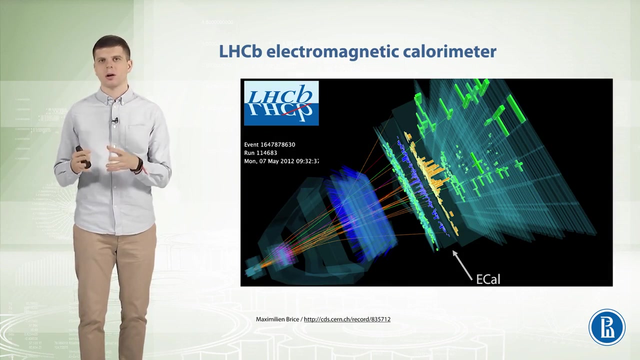 During the colorimeter calibration process In the LCB detector. a lot of these crystals are collected in the matrix. as it's shown on the slide, In the LCB detector model the electromagnetic colorimeter responses are represented as blue columns. One particle can activate several crystals of the 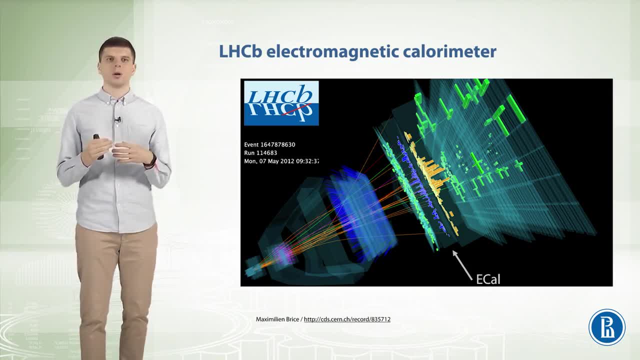 colorimeters. Thus it's needed to recognize a crystal cluster corresponds to a particle to estimate the particle energy more precisely. To do this, a particle track estimated in the tracking system is extrapolated to the electromagnetic colorimeter. Then crystals close to the track in the 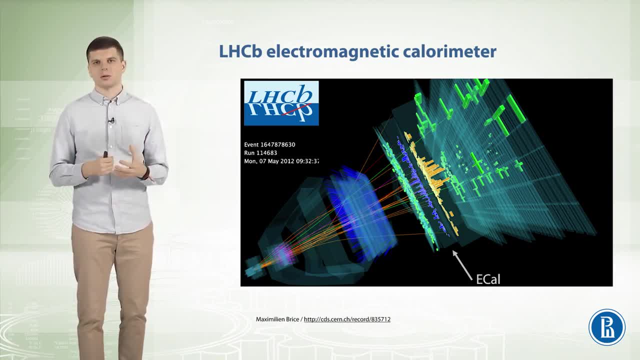 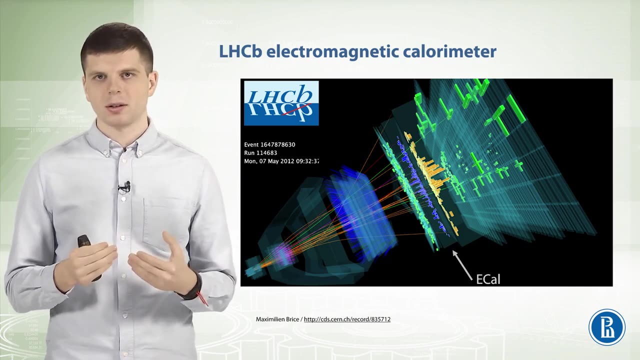 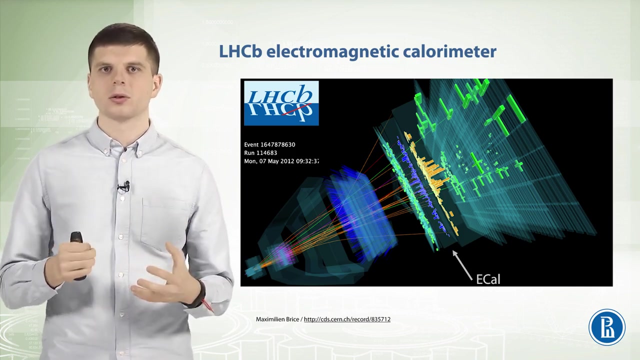 colorimeter are grouped into a cluster and sum of energies measured in all crystals of the cluster corresponds to the particle energy. Machine learning approaches can be used to recognize these clusters and estimate the particle energy more accurately. Moreover, photons are also create clusters in the colorimeter, but they know heats in the tracking system and their tracks are not. 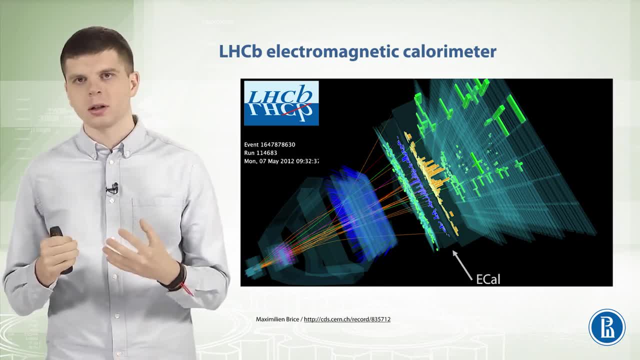 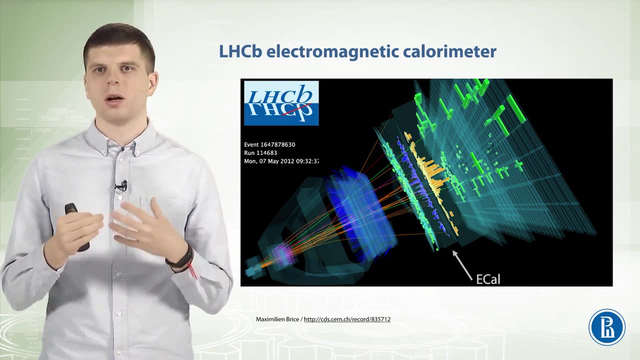 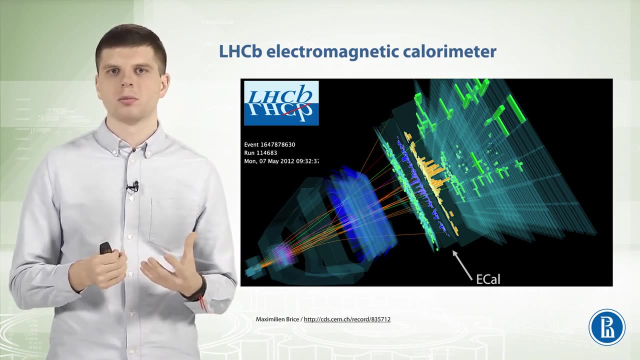 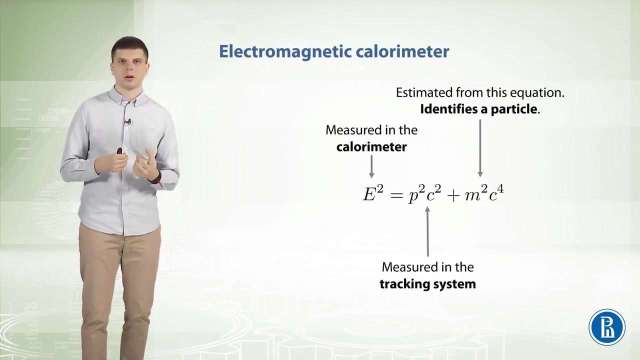 recognized. So machine learning can be used to recognize clusters for photons and separate them from clusters for electrons, Electrons or just noise clusters. So electromagnetic colorimeters are also responsible for photons detection. Consider how colorimeters help to identify particle types. The equation of the slide represents the connection. 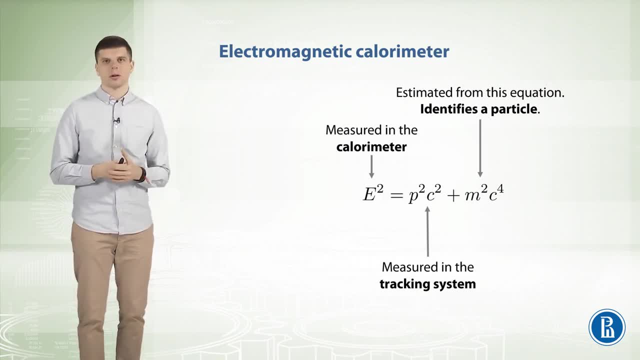 between energy, momentum and mass of a particle. We already know that the particle energy is measured by colorimeters. The particle energy is measured by the colorimeters. In the previous videos we see that momentum of the particle is measured by tracking systems. So, using this equation, we can estimate the particle mass and, as 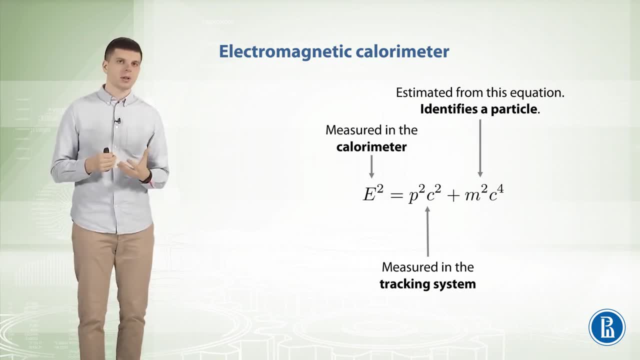 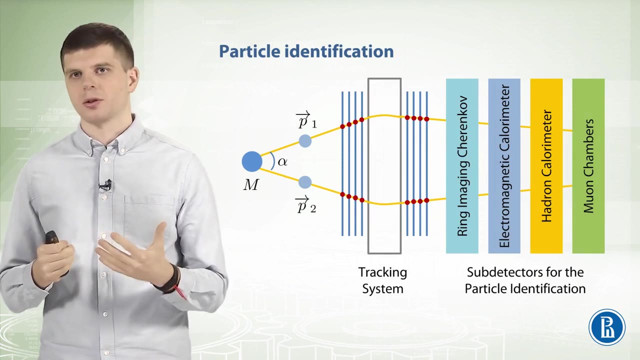 a result, its type. However, in the next videos who, we will see how to use information from all detector systems to identify particle types more accurate. Now our exercise ends. Thanks for watching. see you in the next one. Now let's talk about the adren colorimeter. 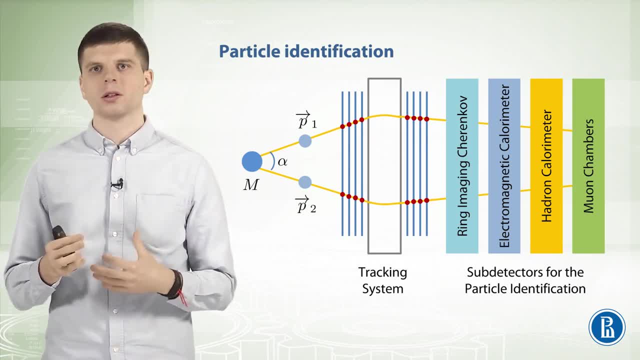 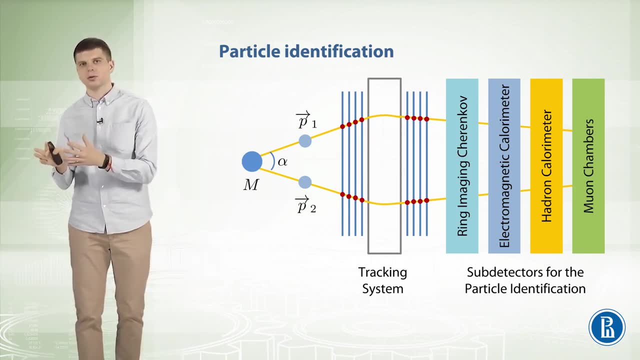 As it was told in the beginning of this video, electromagnetic colorimeter stops electrons and photons. Other particles fly further to the adren colorimeter, And adren colorimeter stops protons, neutrons and other particles containing quarks. In high-end geophysics experiments, adren colorimeter stands after the electromagnetic 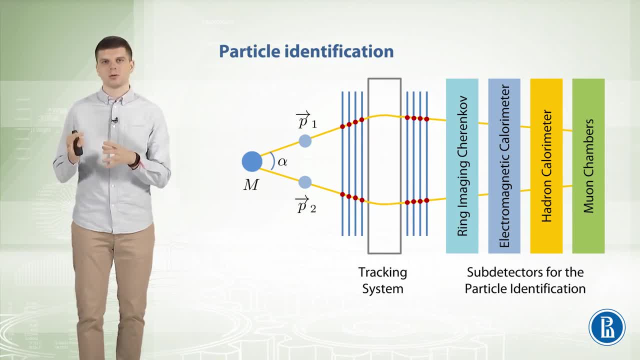 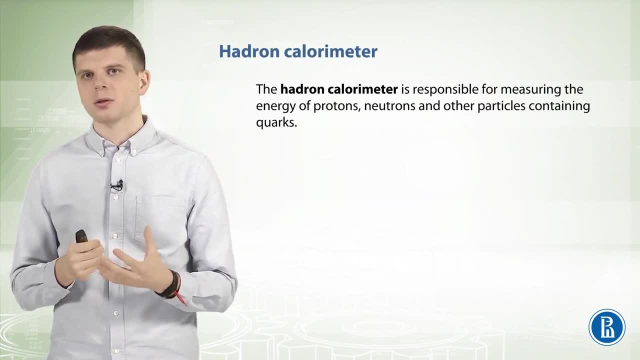 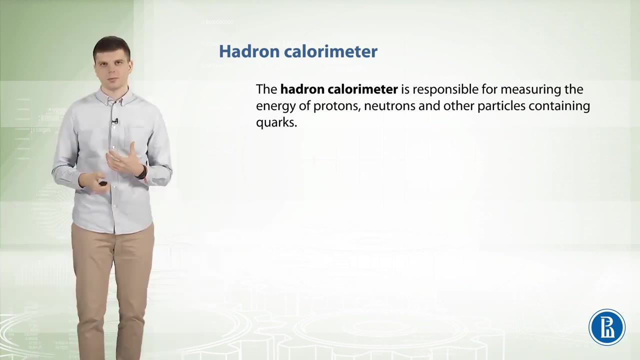 colorimeter. There are only muon chambers after the adren colorimeter, due to muons pass all detector systems. The adren colorimeter is responsible for measuring the energy of protons, neutrons and other particles containing quarks. The principle of the adren colorimeter work is similar to the electromagnetic colorimeter. 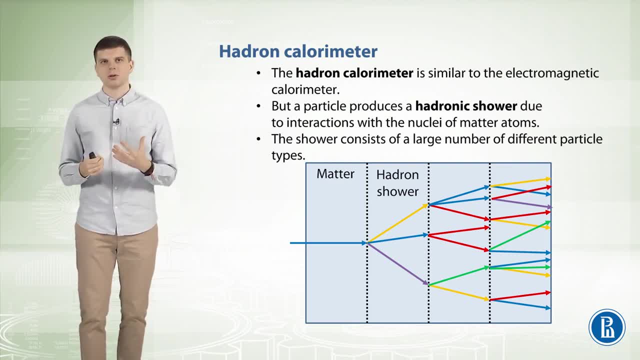 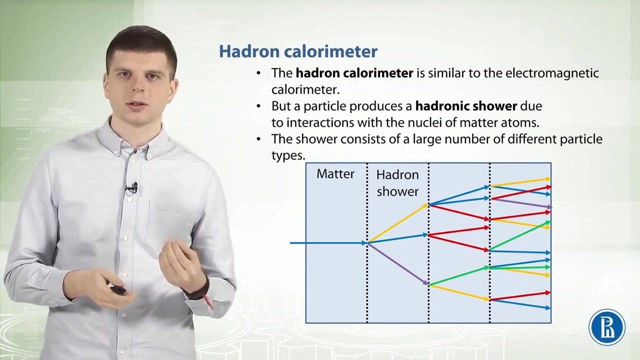 one, But the incoming particle produces an adrenic shower instead of the electromagnetic shower. due to interactions with the nuclei of matter, atoms, This shower consists of a large number of different particle types, not only electrons and photons. The number of particles in the shower exponentially increases with the length of the shower. 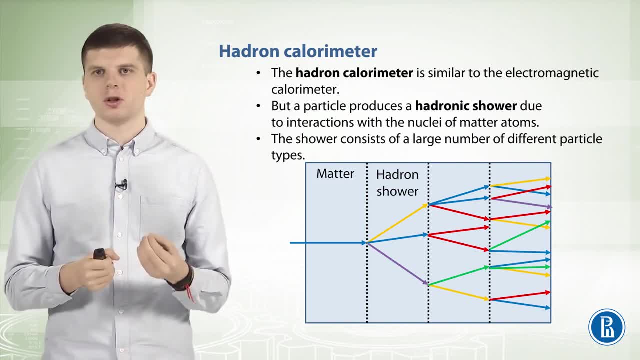 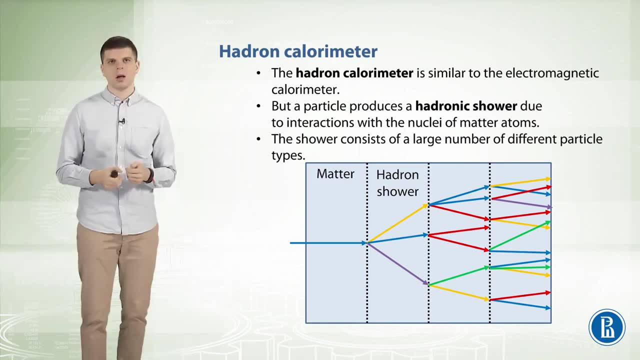 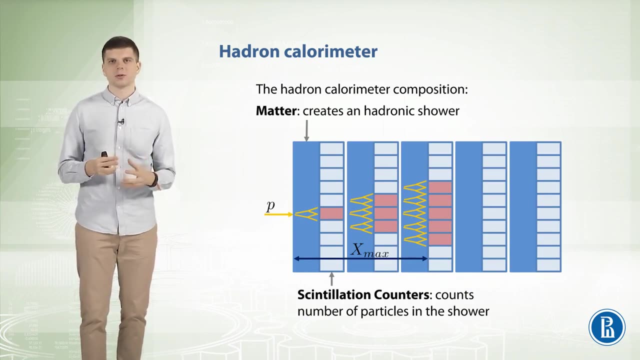 In the same time, the particles in the shower increase exponentially with the length of the shower. In the same time, energy of each particle in the shower exponentially drops, as well as for the electromagnetic showers. Adren showers are larger than electromagnetic one, So the adren colorimeter consists of several layers. 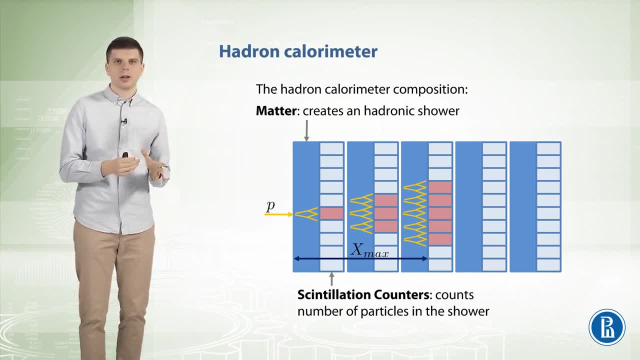 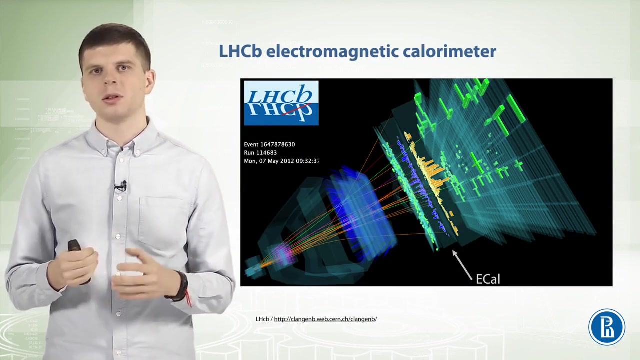 Each layer has a layer of matter that creates an adrenic shower and its installation counter layer that counts number of particles in the shower. Unlike electromagnetic colorimeters, adren colorimeters use heavy materials such as metals. In the LHTB detector model, the adren colorimeter responses are represented as orange cells. 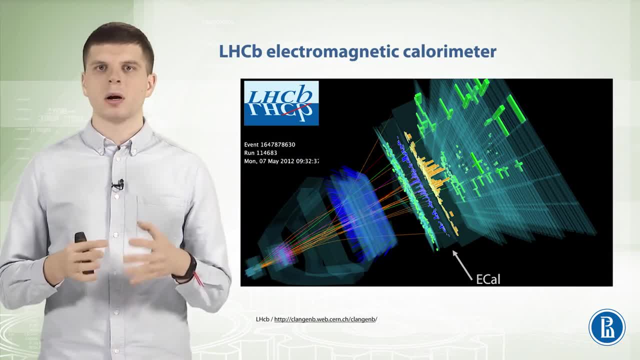 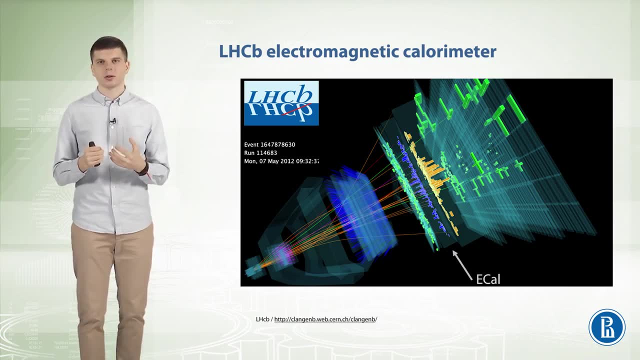 Similarly to the electromagnetic colorimeter, one particle can activate several cells of the colorimeters. Thus, it is needed to recognize a cluster of cells corresponding to the colorimeter. The first component of the colorimeter is the electron. The second component is the electron. 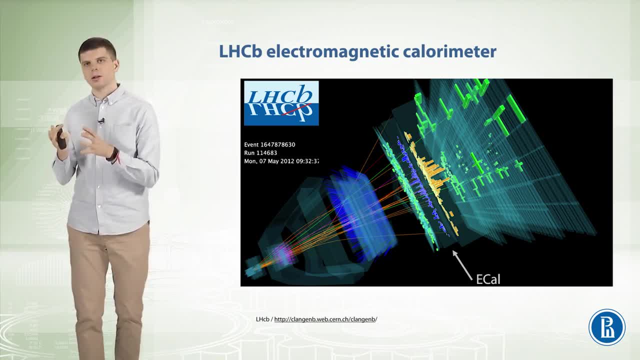 The third component is the electron to the particle. to estimate the particle energy more precisely And to do this, a particle track estimated in the tracking system is extrapolated to the adren colorimeter. Then cells close to the track in the colorimeter are grouped into a cluster. 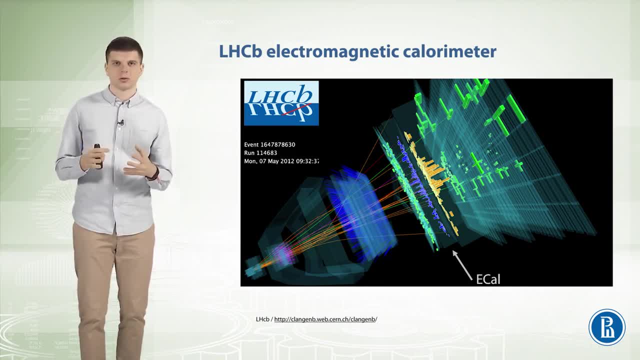 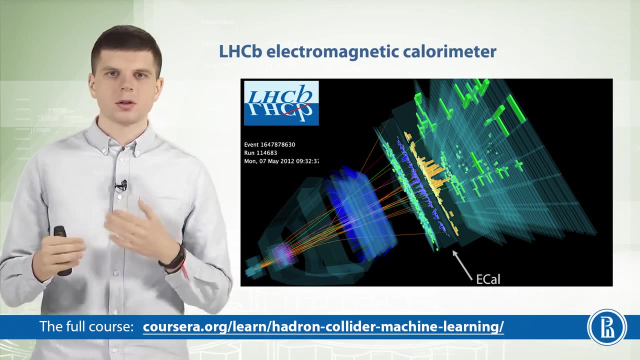 And sum of energies measured in all cells of the cluster corresponds to the particle energy And again, machine learning approaches can be used to recognize these clusters and estimate the particle energy more accurately. This is all about the colorimeters and in the next video we will talk about the last. system of the detector. 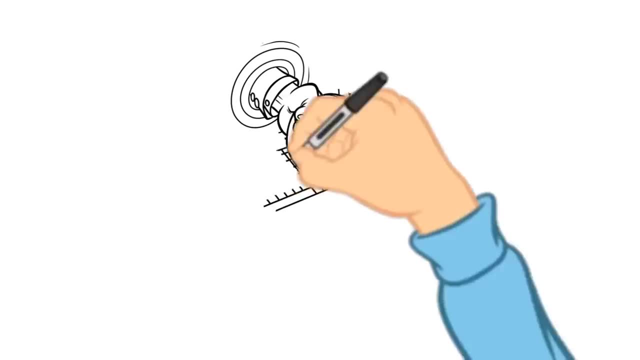 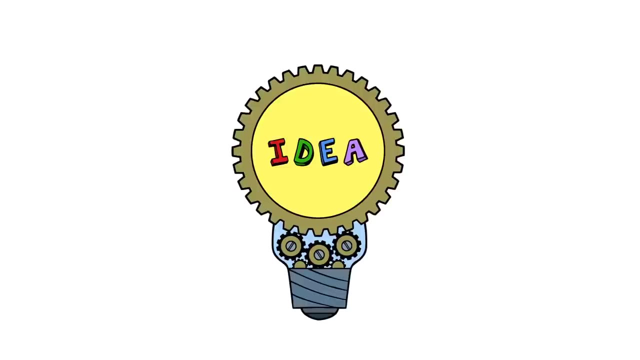 Hey, I know you're about to watch another video, but before you do, I want to show you a cool new software that can grab and keep someone's attention in a super unique way. It's done by drawing literally anything, and I'll show you how anyone can do it regardless. 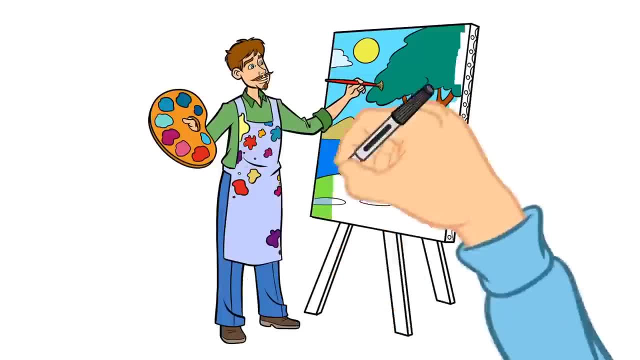 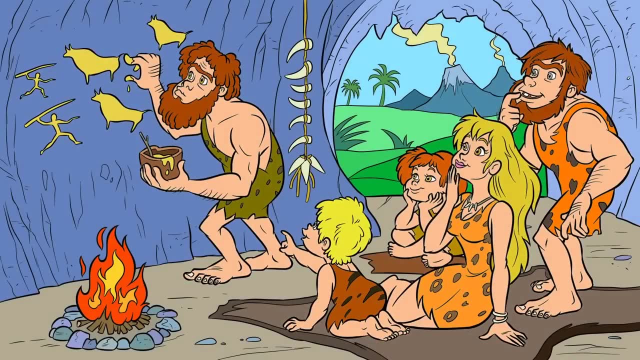 of technical or design skills. As people, we're wired to create as well as watch others create, And by nature, we're also super curious. We tend to want to know and predict what's going to happen next, And this is exactly why we'll sit staring at a screen heavily. 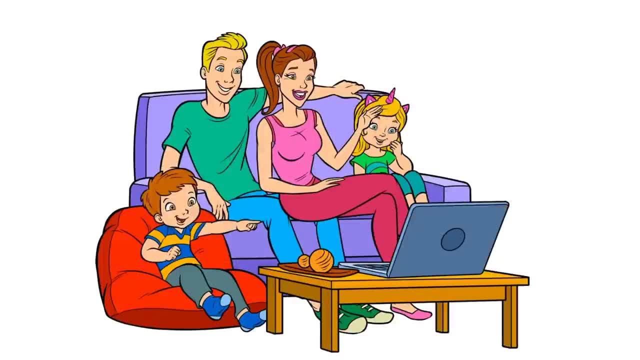 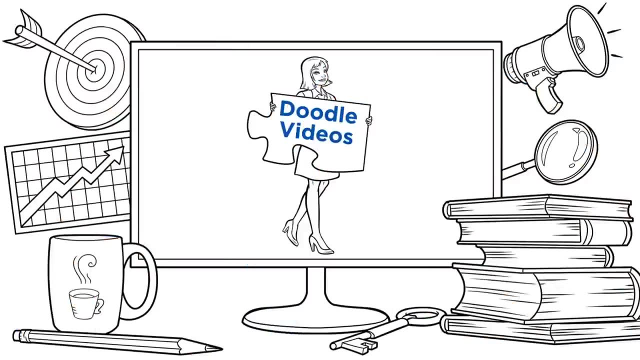 focused on a video just like this in order to see what's going to happen or be drawn next. This is called a doodle video and it's one of the very best ways to engage, teach, sell and entertain an audience. Hi, I'm Brett Callan, and in this video I'm going to show you how anyone can quickly and 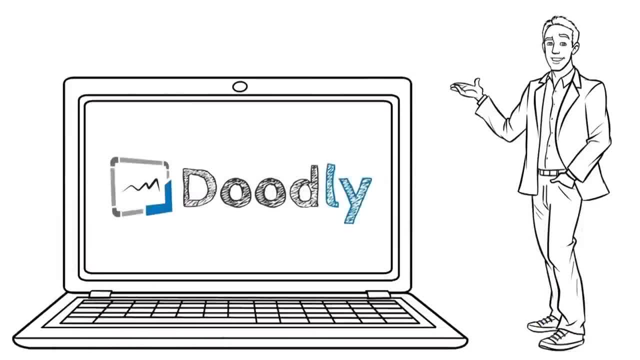 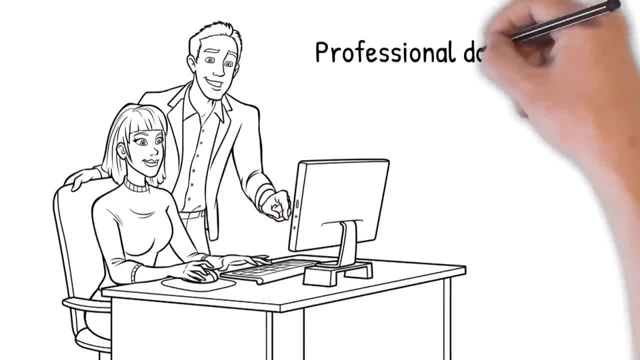 easily create doodle videos, just like the one you're watching right now, using Doodly, our drag and drop doodle software that allows anyone, regardless of tech skills, to create highly engaging professional doodle videos in a matter of minutes. Because doodle videos?